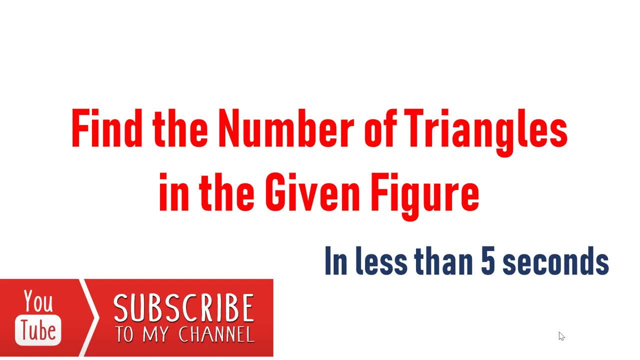 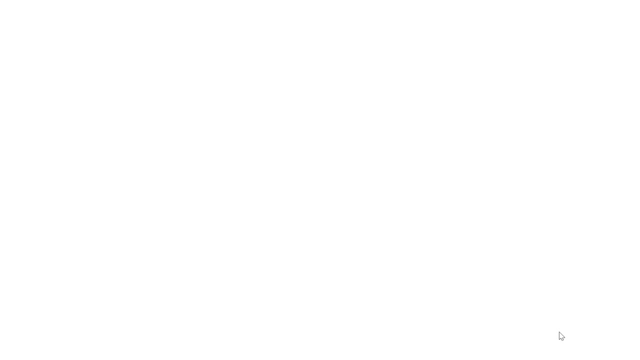 also within triangle itself. I will teach you how to count number of triangles in any figure within 5 seconds. Do watch the complete video for maximum utilization. Everyone must remember that different tricks are applicable to different patterns, so remember the tricks properly. Let's go type by type. 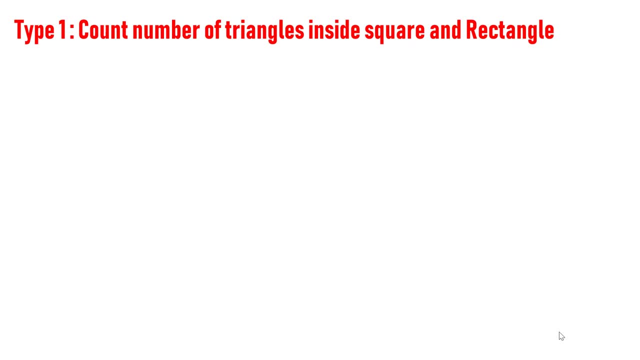 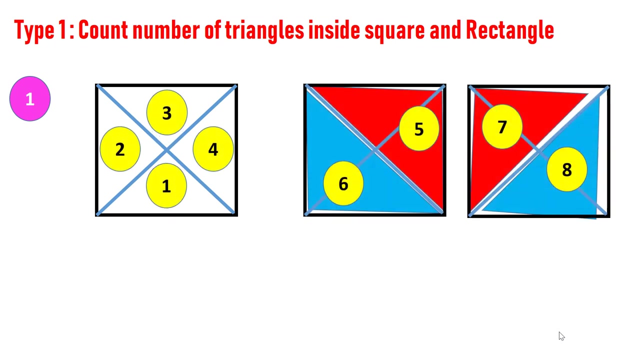 In type 1, let us understand how to count number of triangles inside square and rectangle. First, count number of triangles manually. Later we will take the trick to count number of triangles. Here you can count the numbers manually. In this instance you can count the number of the triangles with me. 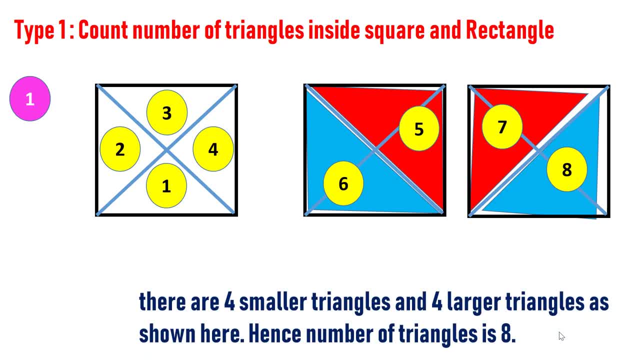 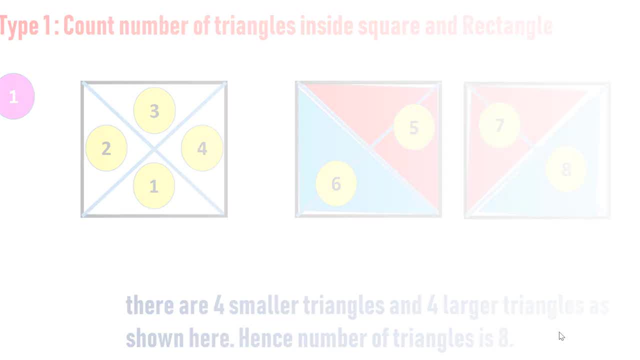 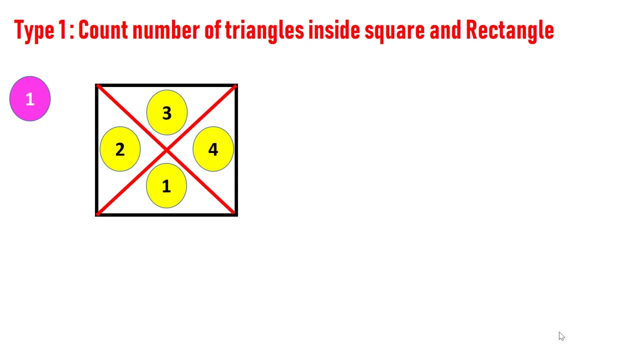 and 4 larger triangles, as shown here. Hence number of triangles is 8.. You need not to count the triangles like this. The trick in this figure is there are 2 diagonals and 4 blocks. Just multiply number of diagonals with number. 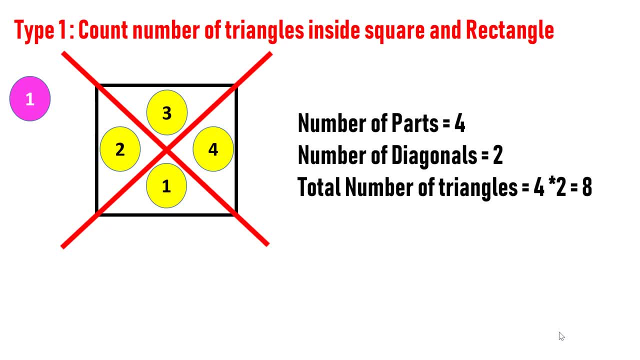 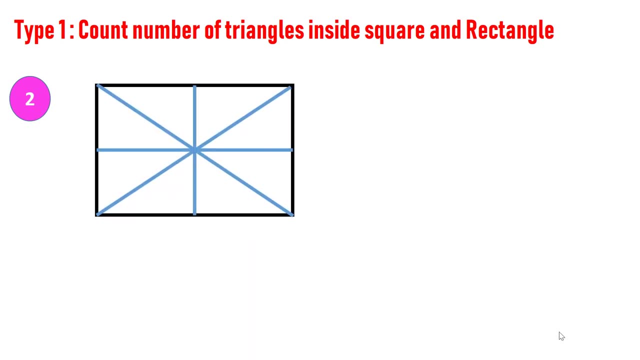 of blocks, Total number of triangles becomes 4 x 2, which is 8.. This is exactly the same number of triangles we got when counted manually. Consider one more figure. in this figure, apply the same trick. Here, number of blocks is 8, and number of diagonals are 2,, 3,, 4, & 4.. This is one more figure in number of blocks, which is 8.. Consider one more figure in number of diagonals, which is 8,, 3,, 4, & 4.. Here, number of block crossed by 3, number. 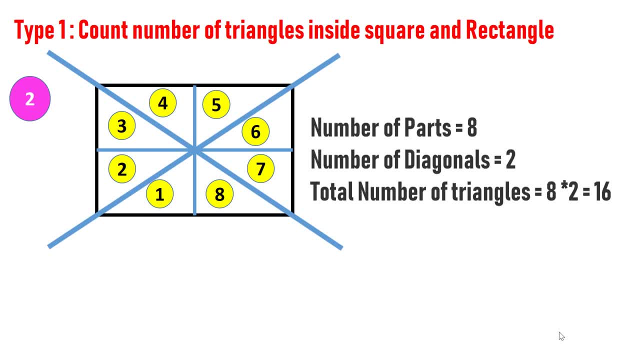 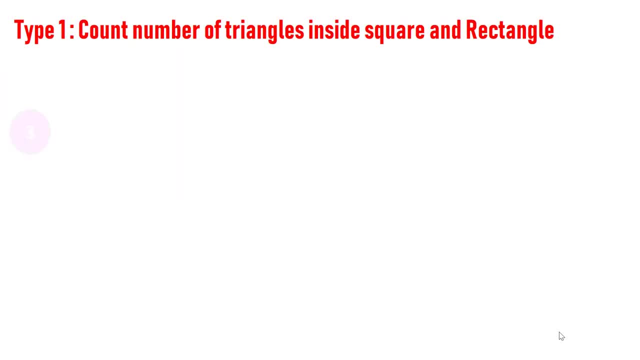 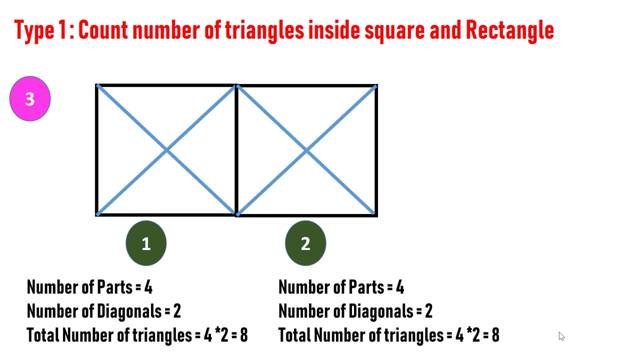 of hurry'قةN' &'a' enforcement: 3, number of loud Taiwaneseuggles: 2. hence, total number of triangles becomes 8 x 2, which is 16.. In this figure, there are 2 squares, and each square has 2 diagonals and 4 blocks. 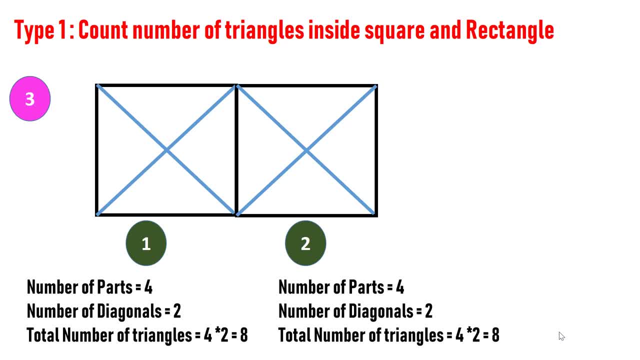 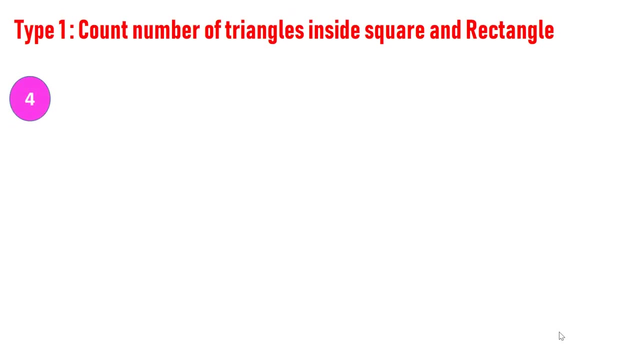 Hence, total number of diagonals in each square is 4 x 2, which is 8.. Also, containing 2 squares will yield additional 2 triangles, as shown here. Hence, total number of triangles are 8 x 8 x 2, which is 18.. 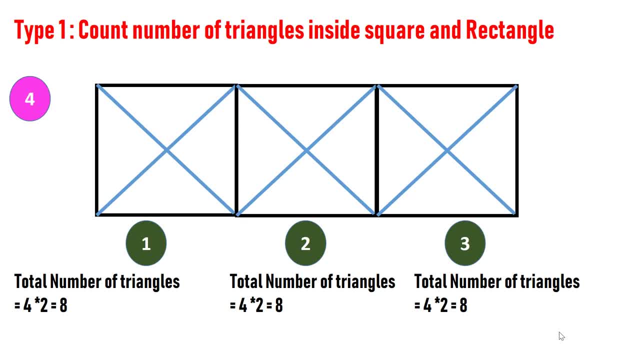 In this figure there are 3 squares And each square has 2 diagonals and 4 blocks. Hence, total number of triangles in each square is 4 x 2, which is 8.. Also containing 3 squares will yield additional 4 triangles, as shown here. 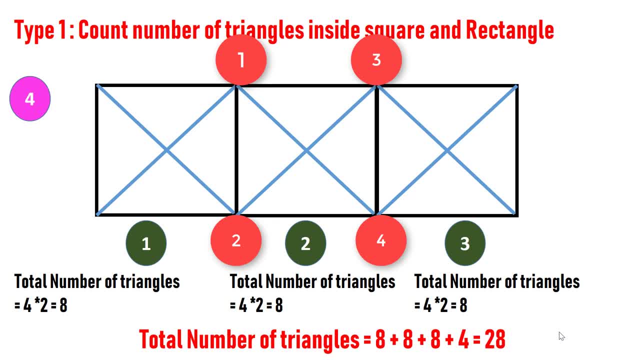 Hence, total number of triangles are 8 x 8 x 8 x 4, which is 28.. Hence, total number of triangles in this figure is 28.. So that's all in type 1.. Let's move on to type 2.. 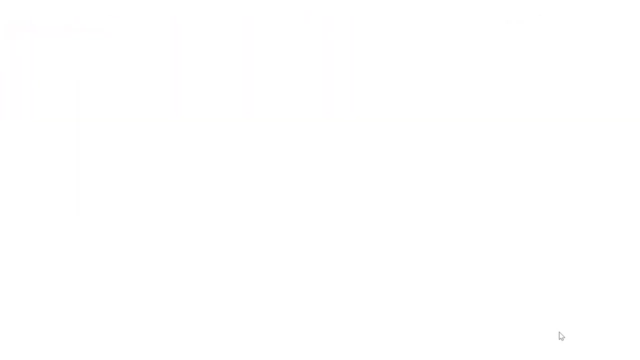 So that's all in type 2.. In type 2, let's understand how to count number of triangles, with a triangle having number of bisects with vertex. So let's consider this figure. In this figure, there is only one triangle and there is no doubt about it. 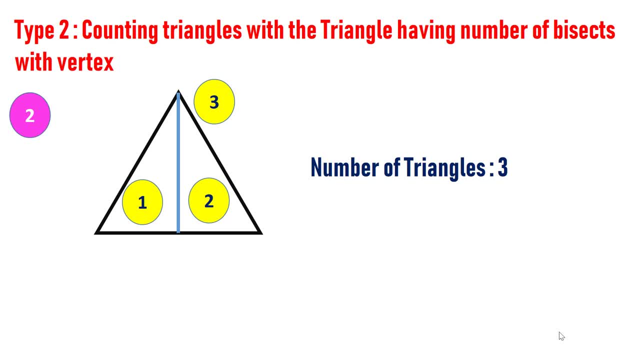 In this figure. if we count number of triangles manually we will get 3 triangles. But this is not the right way to do the counting Because when the figure becomes complex then counting number of triangles manually will not help. Trick here is just number the parts. 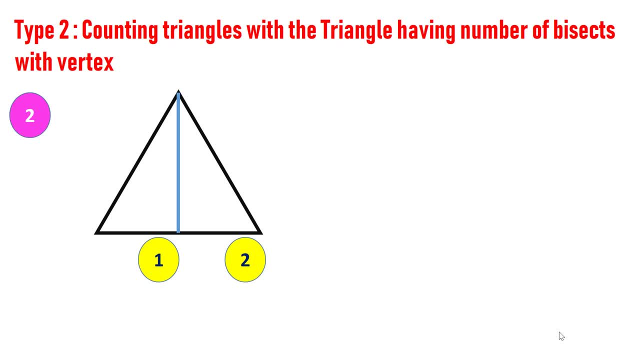 In this figure I have numbered all the parts as 1 and 2.. After numbering, add the numbers. That will be the total number of triangles. In that case, let's look at number 4.. After that, I will tell you how to account for the number of triangles. 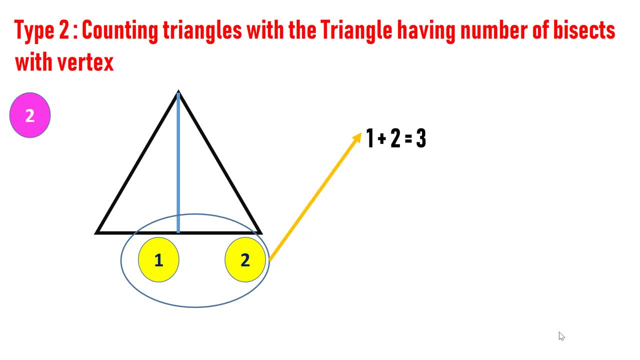 It is possible to calculate them later. I am going to practice number 2 for the 3.2.. here in this figure, adding 192 will yield 3, which is number of triangles in the figure. alternately, you can just count number of parts and multiply number of parts with one number more. 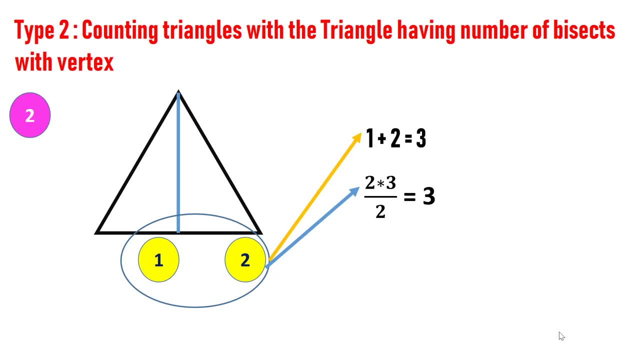 that is, if number of parts are 5. multiply the number with 6 and divide the answer by 2, that will yield number of triangles. let's apply here here number of parts. this figure is to multiply the number with one number more, that is, 3, which will yield 6, and divide it by 2, which will result in 3, which is equal to number. 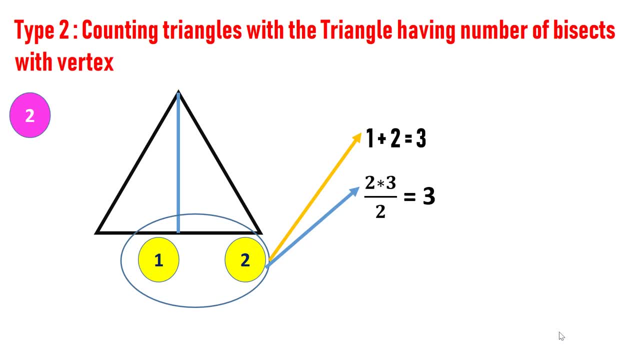 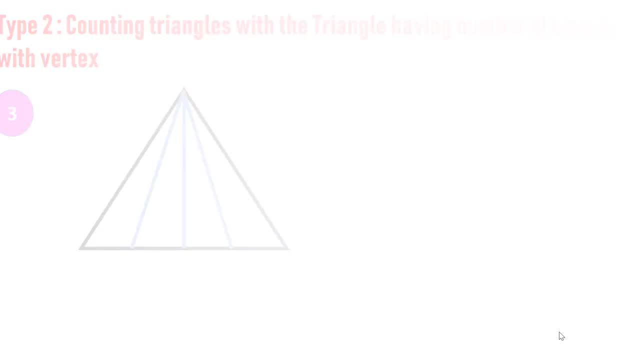 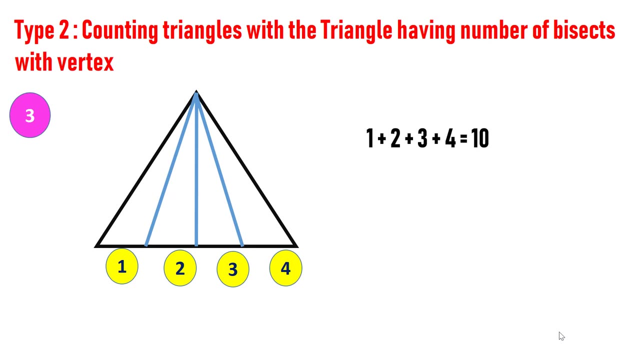 of triangles in this figure. let's consider one more figure: in this figure number all the parts, then add the numbers. hence number of triangles here is 1 plus 2 plus 3 plus 4, which is equal to 10. but if you follow the second trick, number of parts here is 4. multiply this number with one. 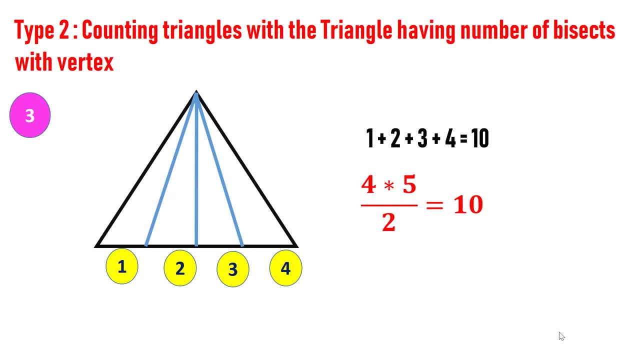 number more, that is 5, which will yield 20. then divide it by 2, which will yield 10, so both procedures will yield the same result. you can use the trick whichever you are comfortable with. remember. second trick is nothing but indirect, using some of all natural numbers. the formula is n into n plus 1, divided by 2. 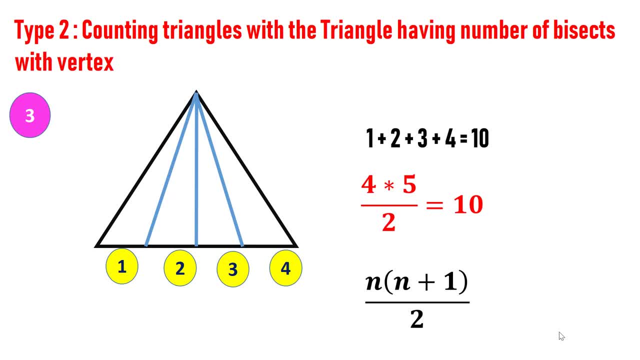 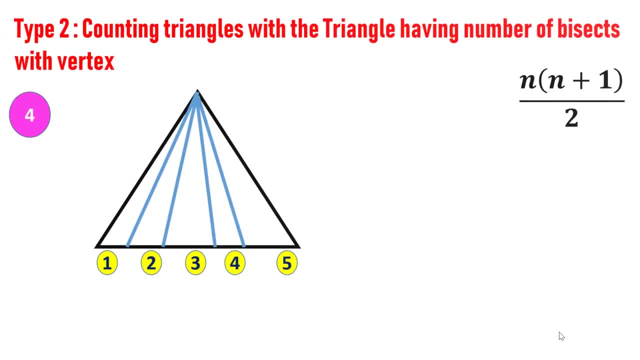 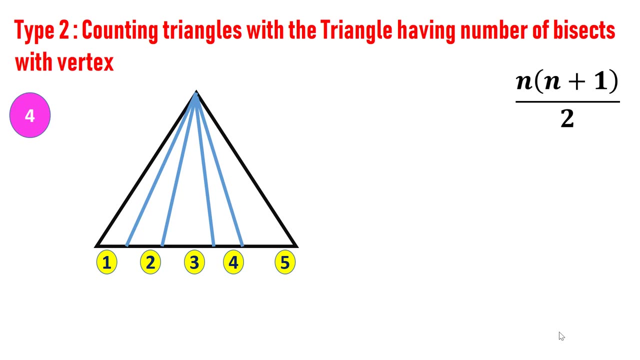 we are exactly using the same formula indirectly. consider one more example. so this is a pretty complex figure. let's apply the second trick here. number of parts are 5. multiply this with 6, which will yield 30, and divide it by 2, which results in 15. so number of triangles in this figure is 15. 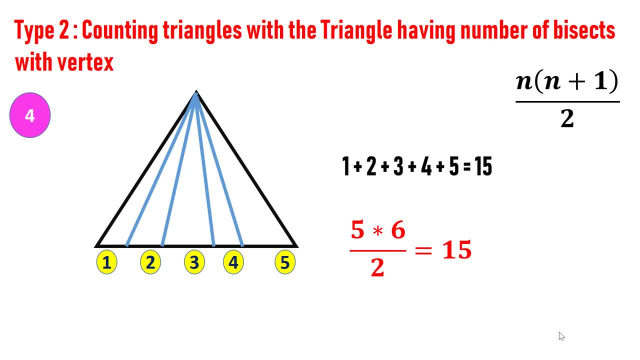 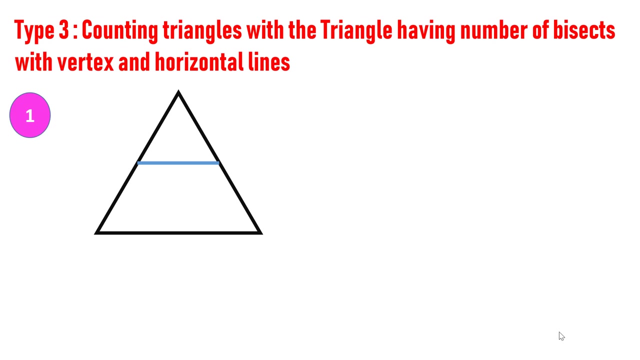 try both the tricks and share which one you feel better in your opinion in the comment section. so that's all in type 2. let's move on to type 3. so in type 3, let's understand how to count number of triangles, with a triangle having number of bisects, with vertex and horizontal lines. so in this, 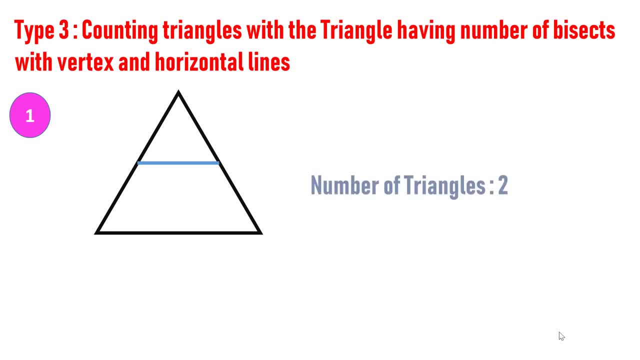 figure. there is no need of any trick. we can just count number of triangles. we can just count how many triangles are there in this figure. there are only two triangles in this particular figure. let's consider another example. in this figure let's count number of triangles manually. there are six triangles here. but this is not the correct way of approaching the problem. 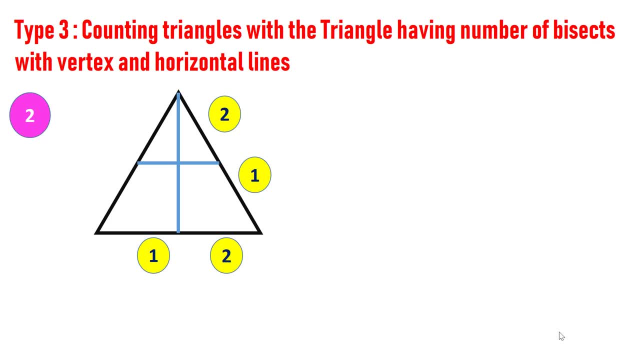 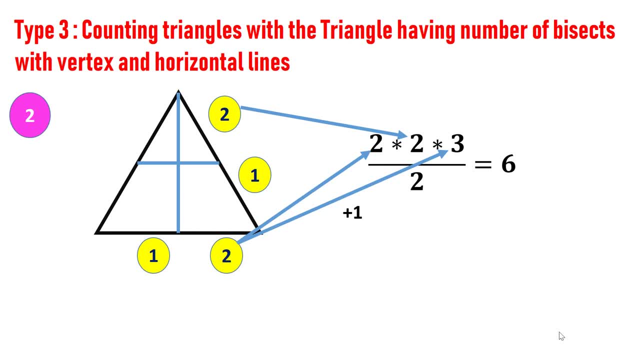 horizontal parts, that is, number of horizontal parts here is 2, and hence multiply the solution with 3, which will yield 12, and divide the solution by 2, which will give you the number of triangles. here it is 6.. Let's apply the trick for little complex figure. 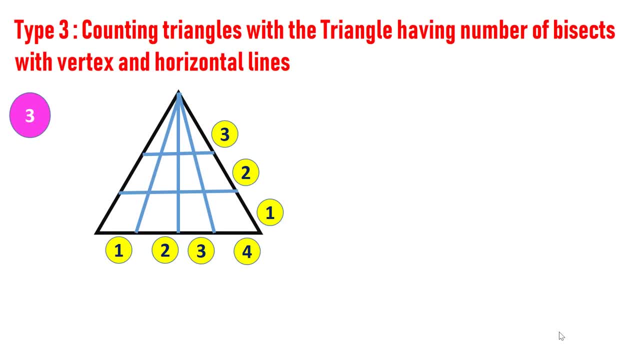 Here, number of horizontal parts are 4 and number of vertical parts are 3.. Multiply, along with the number 1 more than the number of horizontal parts, that is, 4 into 3, into 5, which will yield 60, and divide the number by 2, which will yield 30.. 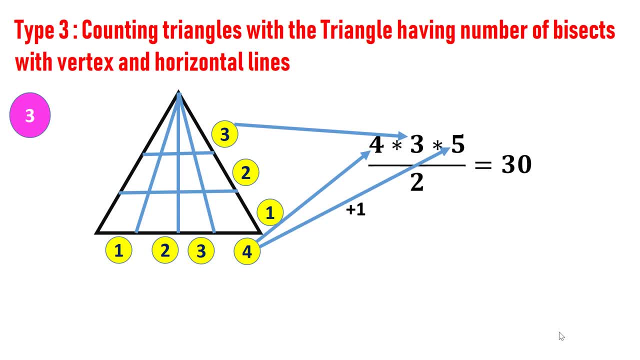 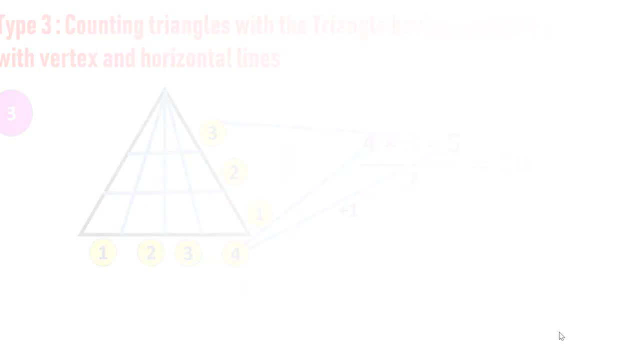 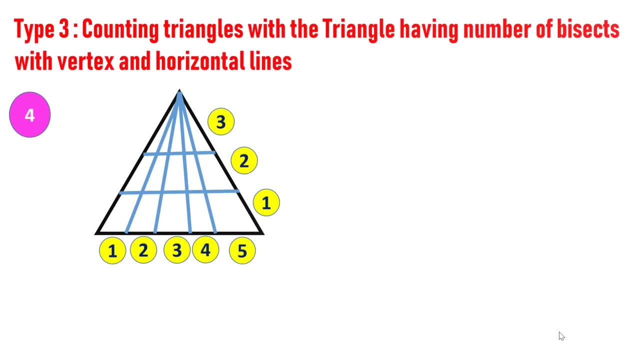 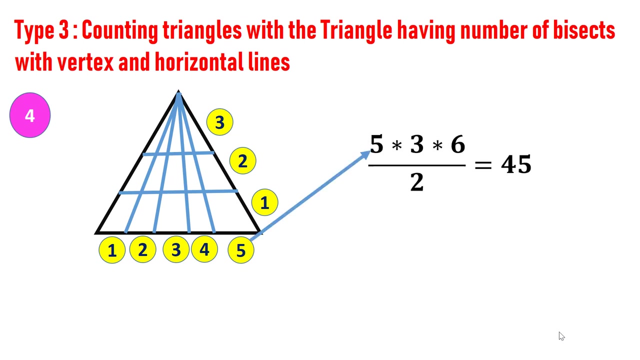 So there are 30 triangles in this figure. By using this simple trick, you can count how many triangles are there in this complex figure. So let's consider one more complex figure. In this figure, number of horizontal parts are 5 and number of vertical parts are 3.. 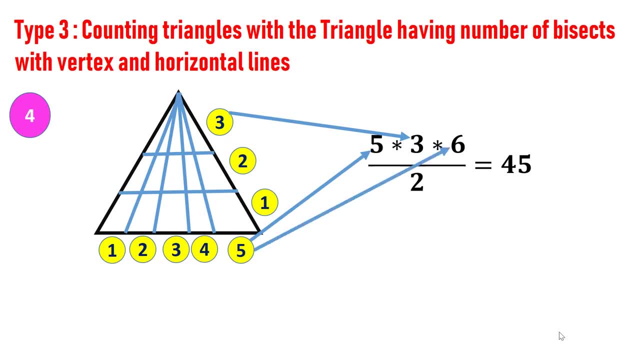 Multiply, along with the number one number more than the number of horizontal parts, that is, 5 into 3, into 6, which will yield 90, and divide the number by 2, which will yield 45. There are 45 triangles in this figure. Now let's try the first of the three triangles. Now, at this point, we see that there are 45 triangles, all with 2 triangles. There are 45 triangles and a number of 6births, which are 4 and 5.. In that case, you add 12 of them, so as 0. 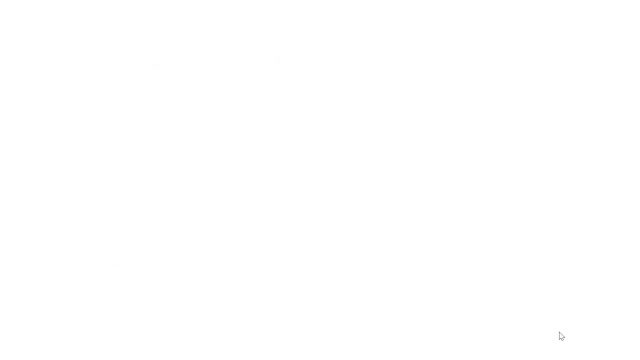 In the next step you have to add 15 of them separately. That's all in type 3, let's move on to type 4.. In type 4, let's understand how to count number of triangles within embedded triangle. So in this type, a triangle is embedded inside a triangle and triangle inside that, and so 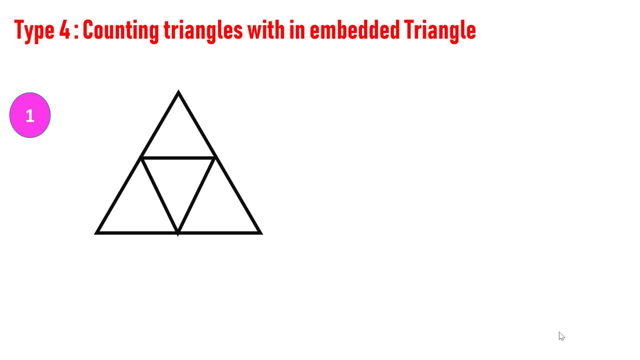 on. Let's understand how to find the number of triangles in such figure. So in this figure we count number of triangles manually. it will yield 5.. Shortcut to find the number of triangles in this kind of patterns is by using the formula. 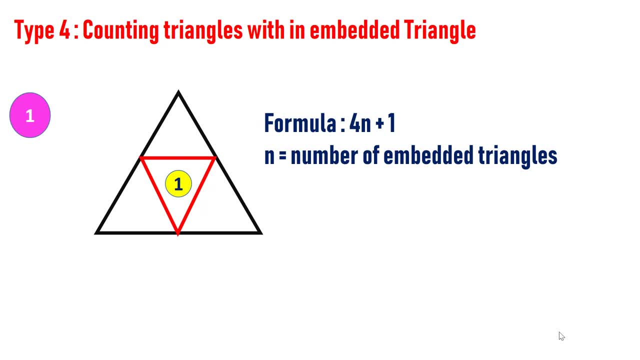 4n plus 1.. Just remember this simple formula to find the number of triangles in this kind of patterns. Here: n is number of embedded triangles In this figure. there is only one triangle embedded, and hence number of triangles in the figure. 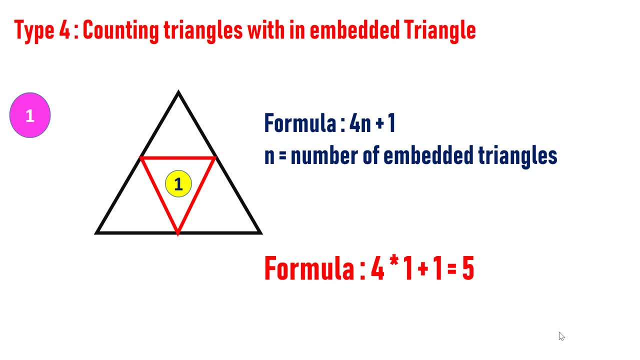 This figure is 4 into 1 plus 1, which is 5.. Let's check the trick with little complex figure. In this figure, number of embedded triangles is 2, hence number of triangles is 4 into 2 plus 1, which is equal to 9.. 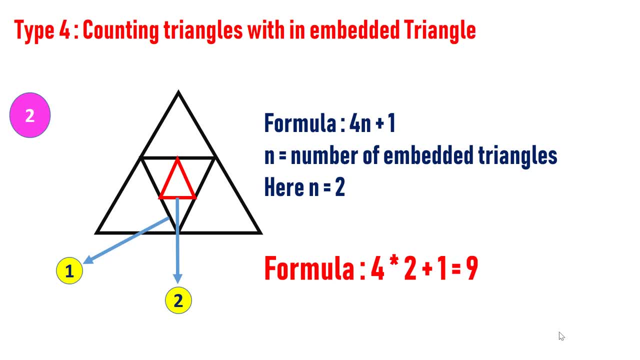 So it is very easy to find the number of triangles in this kind of patterns, if you know the trick. Let's consider one more example. So in this figure, number of embedded triangles is 3.. Hence number of triangles is 4 into 3 plus 1, which is 13.. 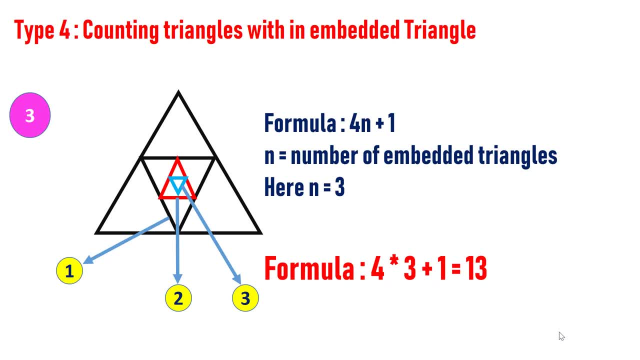 So if you know the formula 4n plus 1,, so if you find this kind of patterns, then apply the formula. So replace n with the number of embedded triangles, you will get the total number of triangles. So if you know the formula 4n plus 1,, so if you find this kind of patterns, then apply. 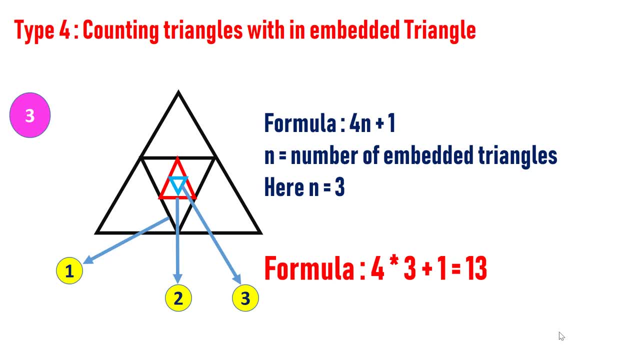 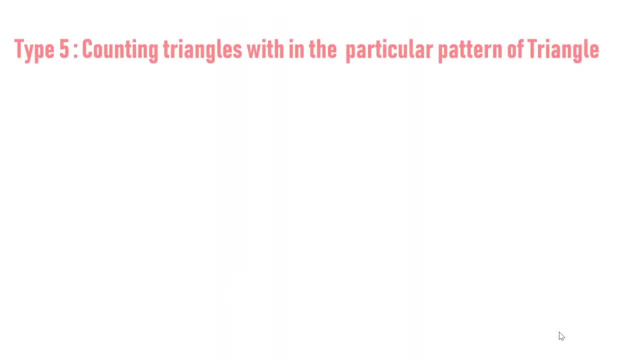 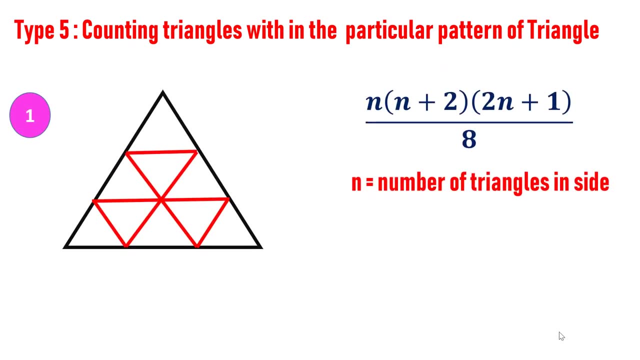 the formula You will get the total number of triangles in this kind of patterns. So let's move on to the final pattern. So in type 5, let's understand how to count number of triangles within the particular pattern of triangle. So these patterns are complex patterns. 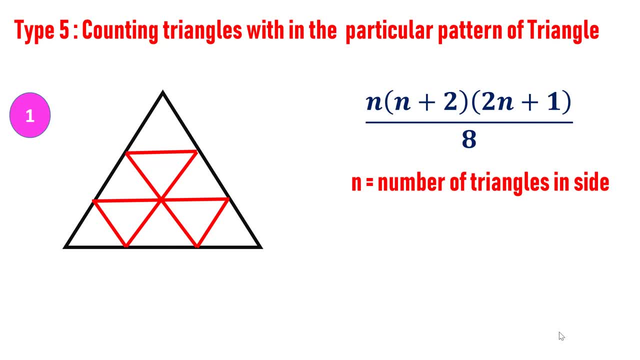 The only trick to find the number of triangles in these kind of patterns is to use the formula. I personally recommend to remember the formula Instead of memorizing a table. formula to count number of triangles for these kind of patterns is n into n plus 2 into 2n plus 1 divided by 8.. 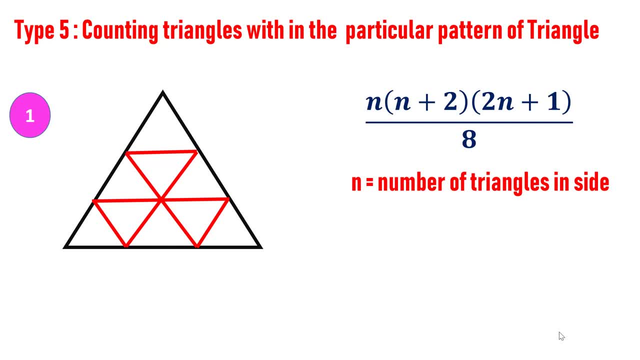 So I will repeat: So formula to find number of triangles in these kind of patterns is n into n plus 2 into 2n plus 1 divided by 8, where n is equal to number of unit triangles in a side. So let's understand this with an example. 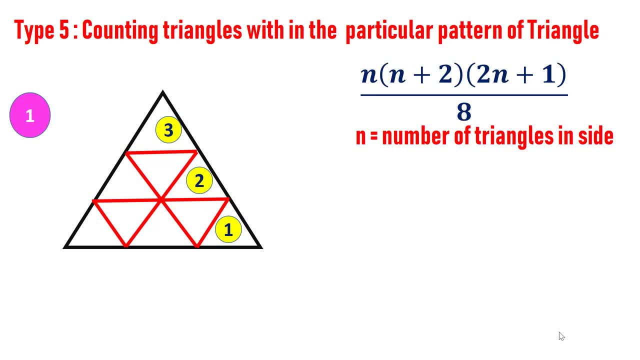 So in this example Number of side triangles in side is 3, use the formula to find number of triangles. In this figure, number of side triangles is 3,, hence n is equal to 3.. Now substituting the value of 3 in the formula, it becomes 3 into 3 plus, 2 into 2 into 3 plus. 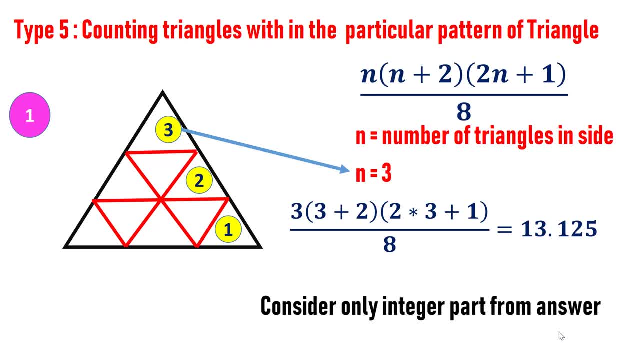 1 divided by 8, which is equal to 13.125.. So number of triangles in this figure is 13.. Note that Consider only integer part from answer obtained in the above formula. For example, the answer may come 13.12. then consider only 13..